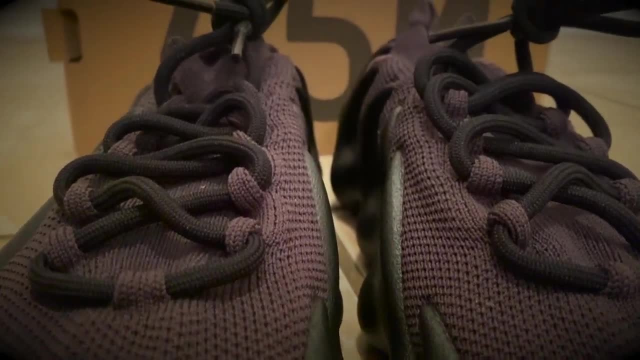 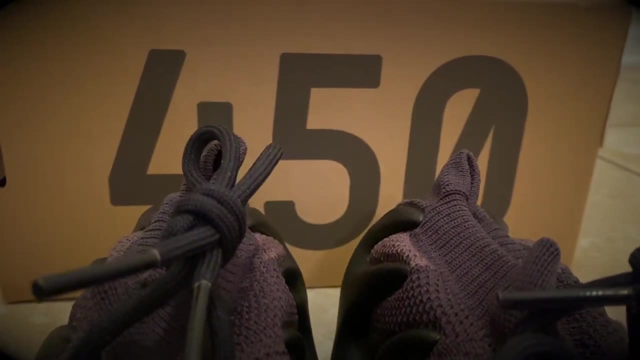 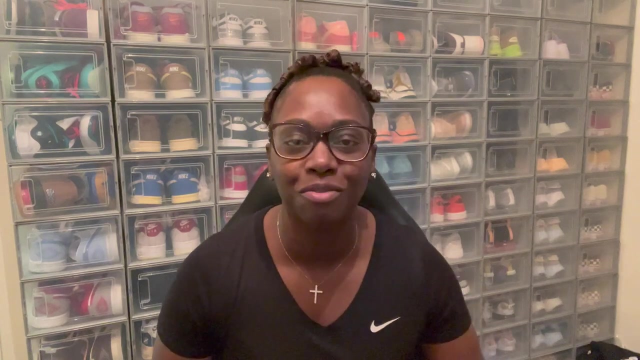 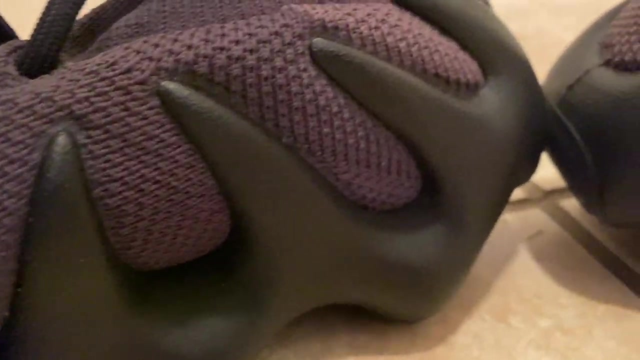 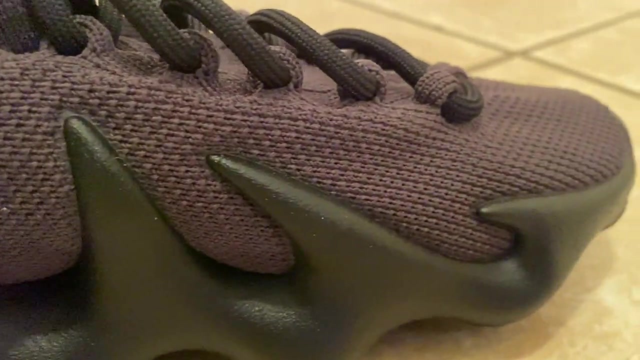 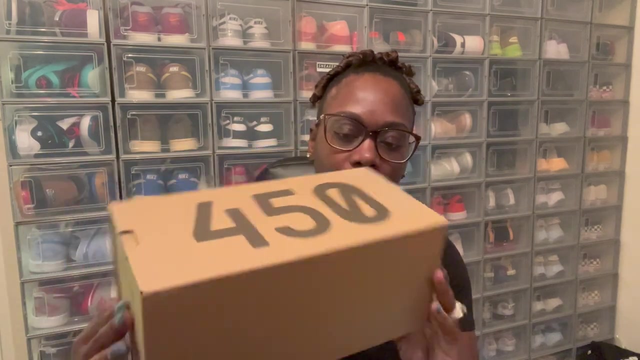 What's going on, everybody? It's your girl, Sneaker Mom, back in the building, back with another review for you guys. Today we're going to be reviewing the Yeezy 450 Dark Slate. Let's get into it First. you got your normal 450 Yeezy box. It says 450 on the top. Now 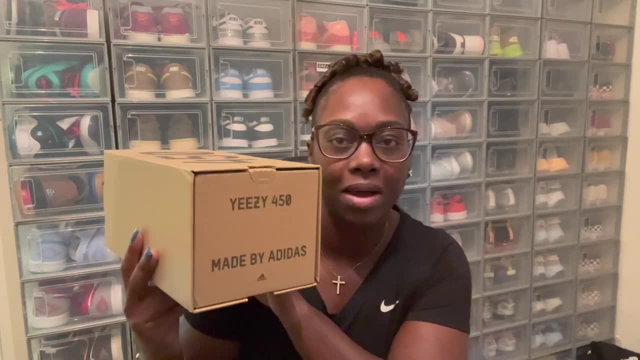 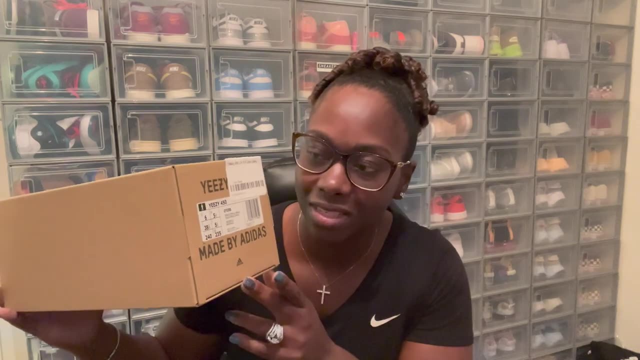 on the sides it says Yeezy 450, made by Adidas, And then the front of the box says Yeezy 450, Dark Slate, Dark Slate, Dark Slate, size 6.. And let's get into it, You're going. 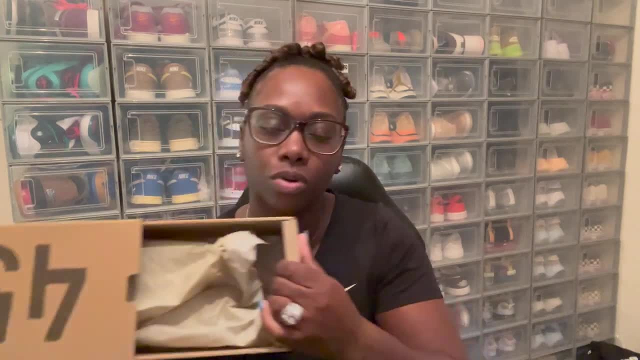 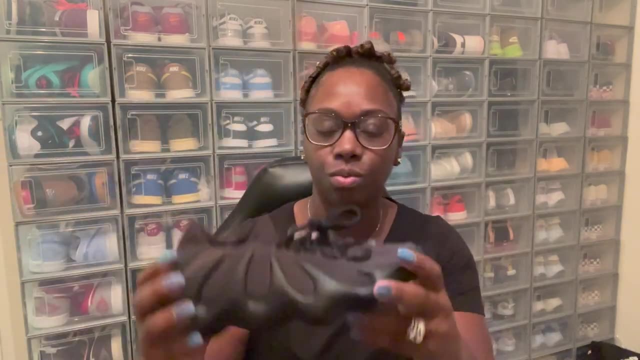 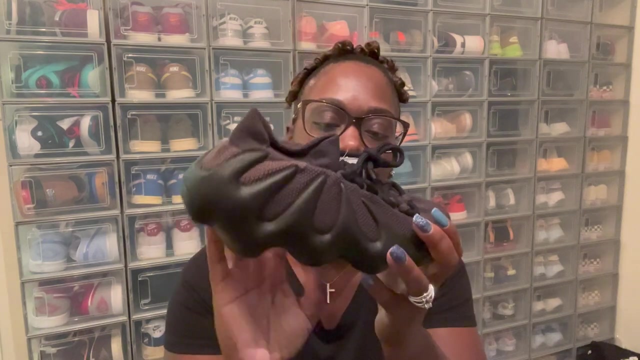 to open the box. You got the same normal cream tissue paper inside the box. Inside that's it. Put that down and we're going to get to the shoe. Here we go. Yeezy 450 Dark Slate. These were restocked on December 17th. That's when I got them on the restock. I'm just getting 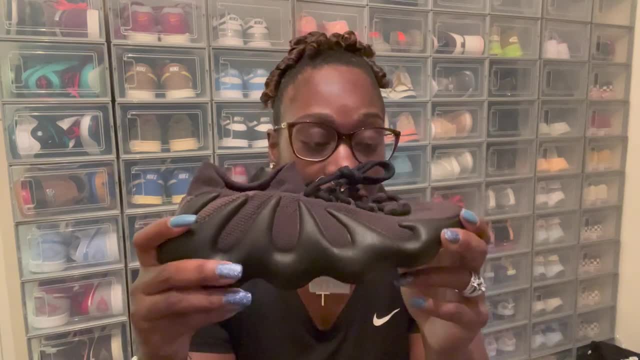 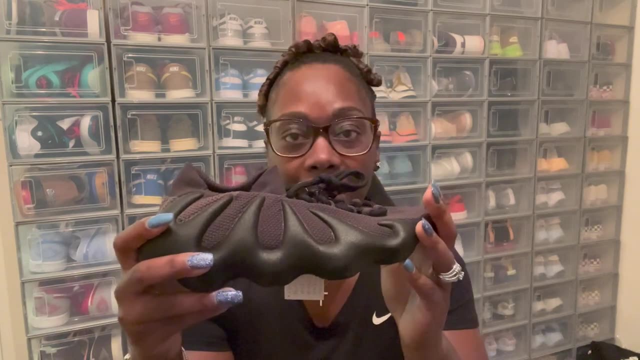 mine in And these were the ones right here. I had the cloud whites but I was like I got to get the dark slates because I assume that these won't get as dirty so fast. I mean because it's all dark And we got to. let's get into the description of the shoe You 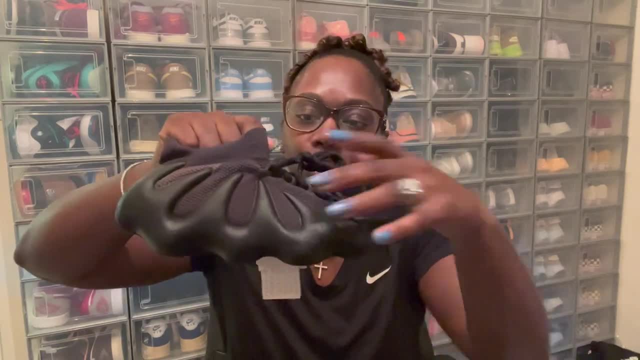 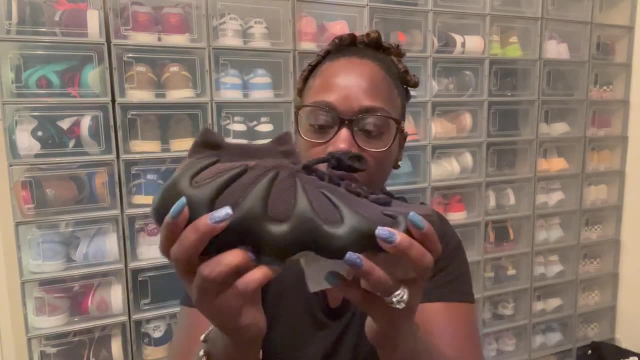 got your all-mesh material going around the shoe. It's a salt-like material, so it sticks. It clings to your foot. real good. You got your rubber- black rubber- going around the shoe that comes up to look like a claw- That's what I would say it look like. You know everybody. 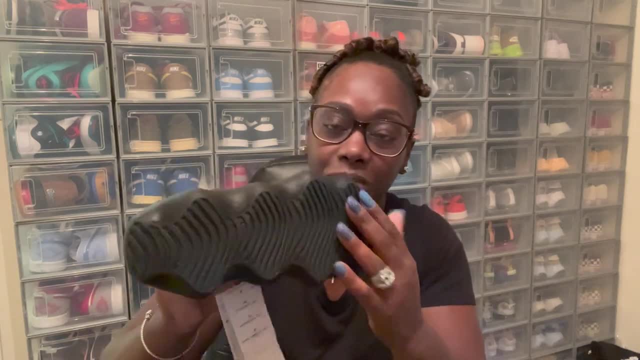 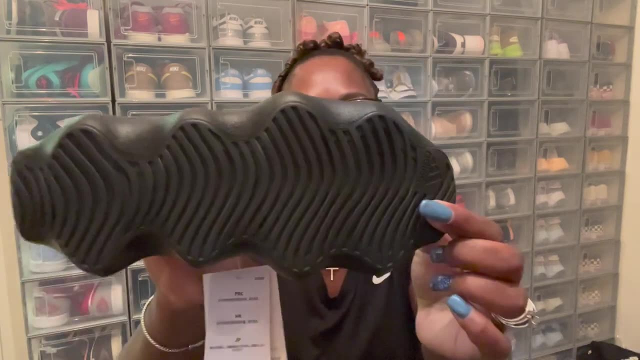 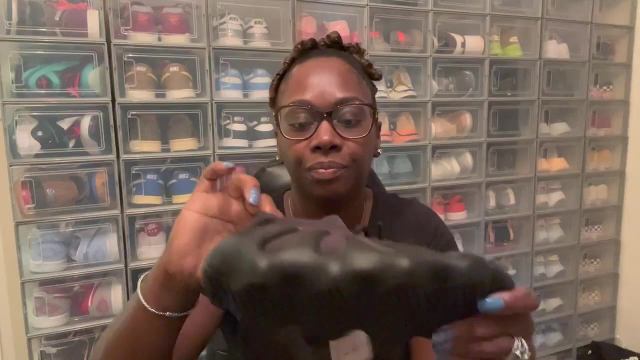 else say it look like dumplings. So we'll go with that. It could look like a claw or some dumplings. You got your black bottom with your little ripple effect going on. that says Adidas on the top of the shoe. right there On the inside of the shoe says Yeezy and it says Ortholite Adidas. I don't know if you 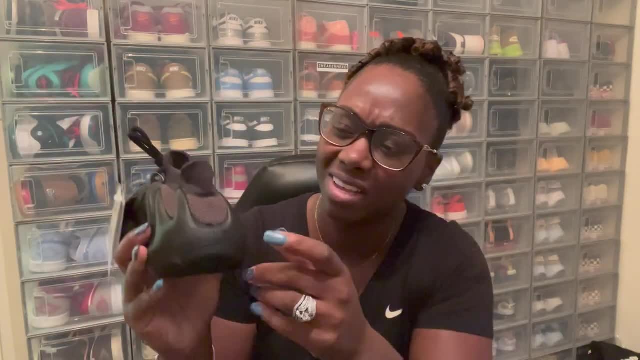 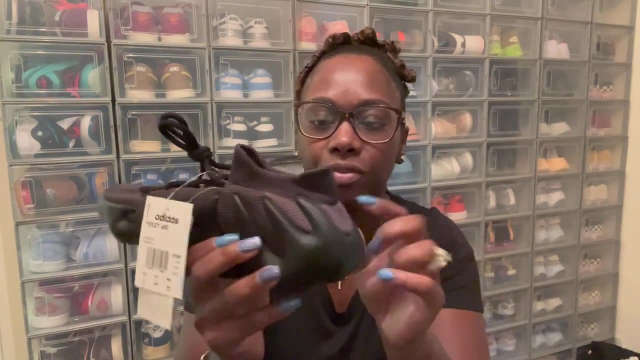 have to see that inside there, In the back of the shoe, it has like a dark brown on the back of the shoe and on the little two sides It's a little different coloring from the dark black, but this could also go as a dark, dark chaco. That's what I would say also. 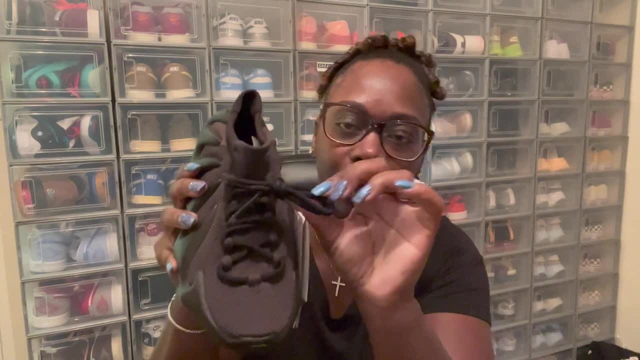 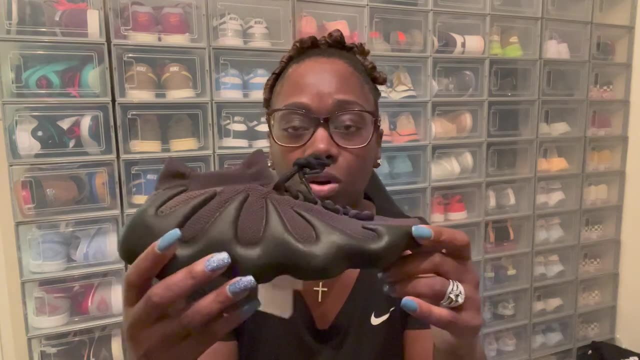 So this would be my dark chaco. And then when you got your shoestring- all black shoestrings- they don't come with any extra shoestrings. The shoestring are really just on the shoe because they really don't do that. Once you put this shoe on, it fits. 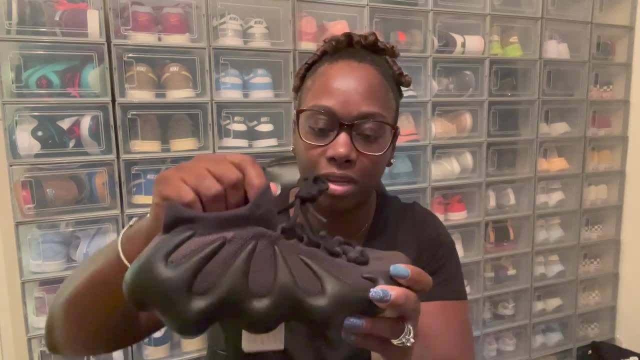 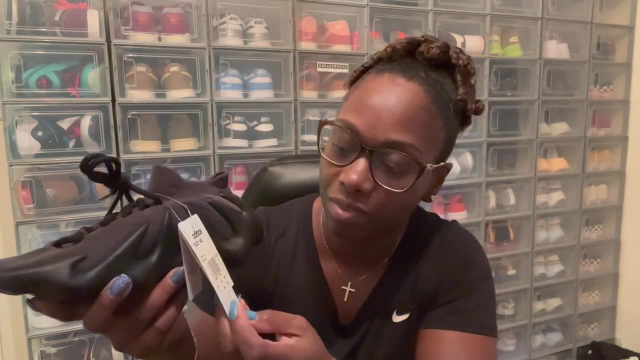 like a glove. So I mean you really don't need the shoestring. So technically they just there for looks. but I mean it makes the shoe look better. It comes with a tag It says Yeezy 450.. Like I said, I got a US size six. That's it for this shoe. This is the. 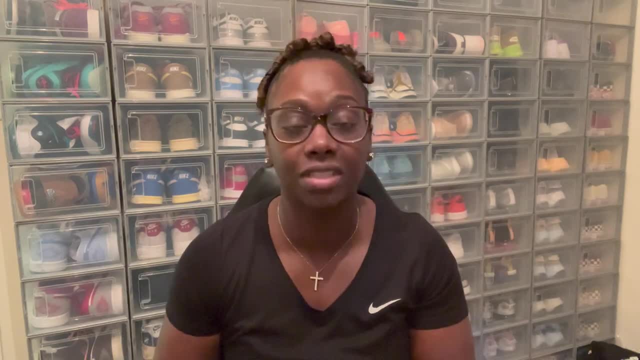 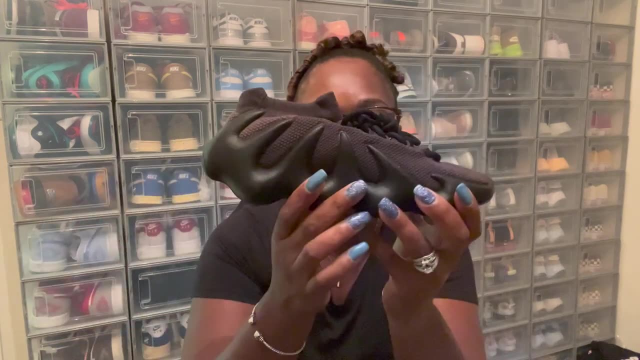 left shoe, Let's get to. oh sorry, That's the right shoe, Let's get to. the left shoe. Looks the same way. You got your black rubber claw doubling look effect going around the whole shoe, Your black ripple effect on the bottom with your Adidas on the top. You got. 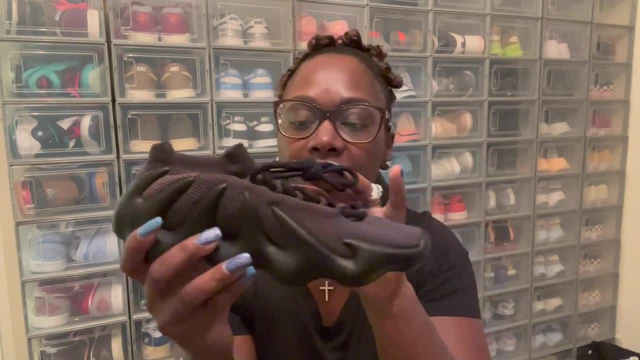 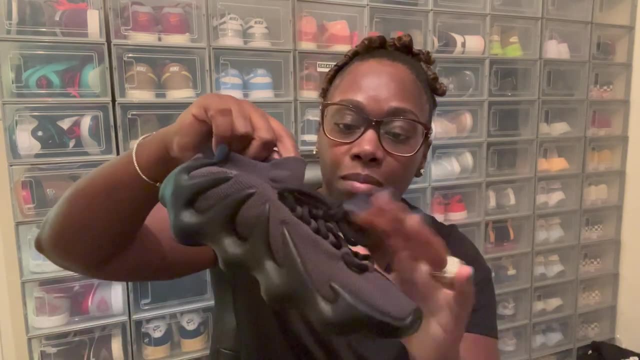 your black shoestrings. and then you got your all mesh, dark, dark gray, or you can call it black, but it looks like a smoke. smoke. gray and your black shoestrings. And then on the inside of the shoe says the same Yeezy, ortho light Adidas. I hope y'all can see the 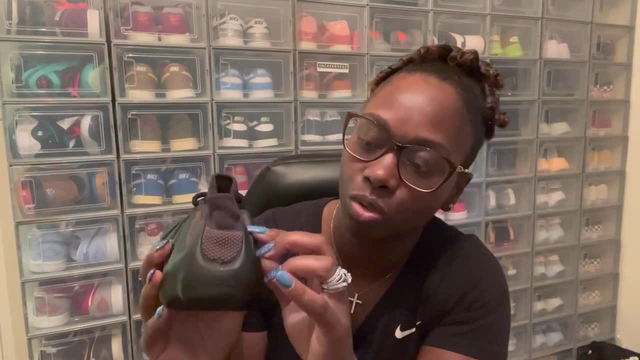 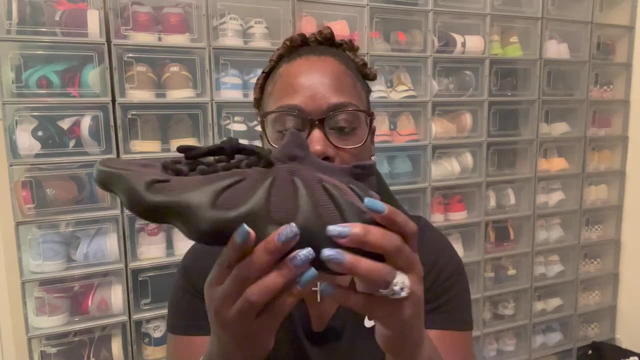 inside of that, The back of it, got your dark brown little speckles on each little piece- I guess it's like the signature for this shoe- to have a dark, a dark brown thing going around the back of it. And you got your ankle area with all salt like material. So once you put your 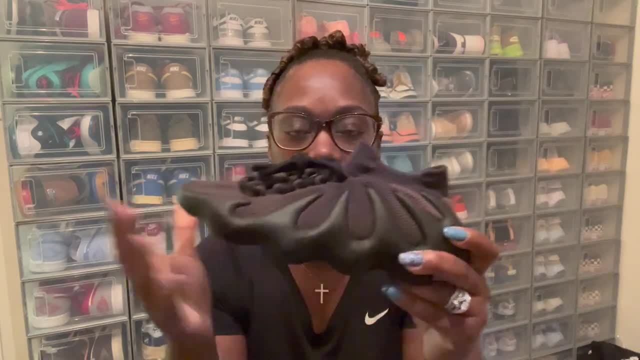 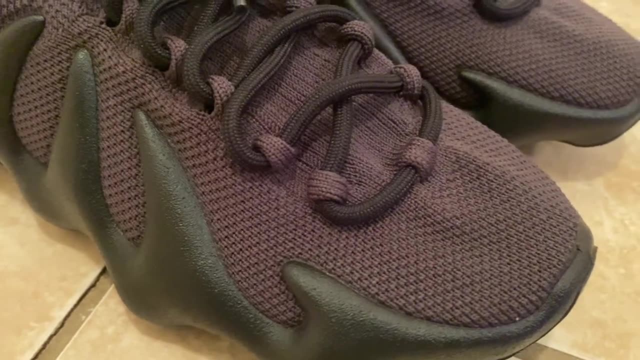 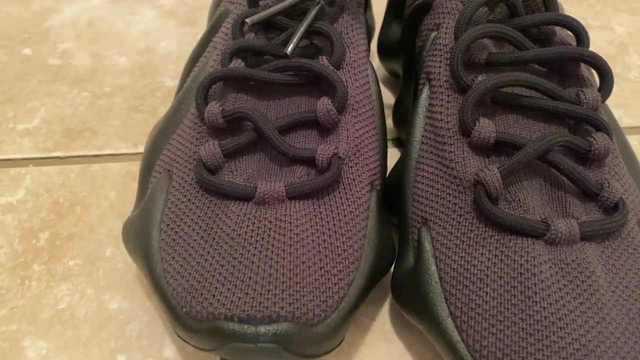 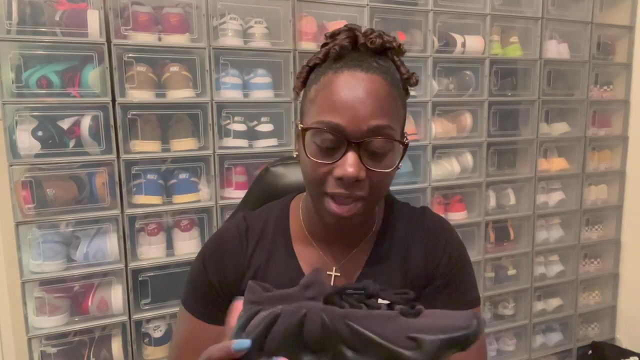 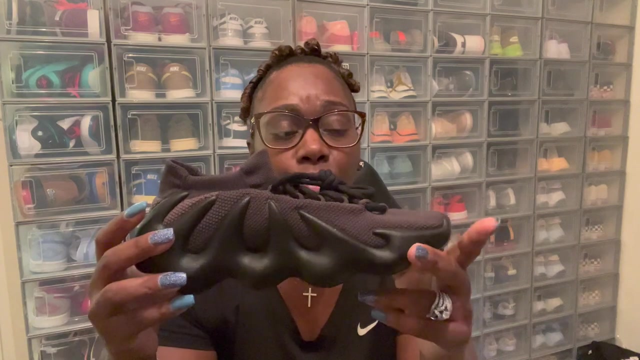 foot in, pretty much locked in. you don't have nothing else to worry about. It's on your foot, Solid shoe. And yeah, these are it. right here I had the cloud whites. like I said, these are the dark slates. I was so excited to be able to get these because they're dark And I'm quite 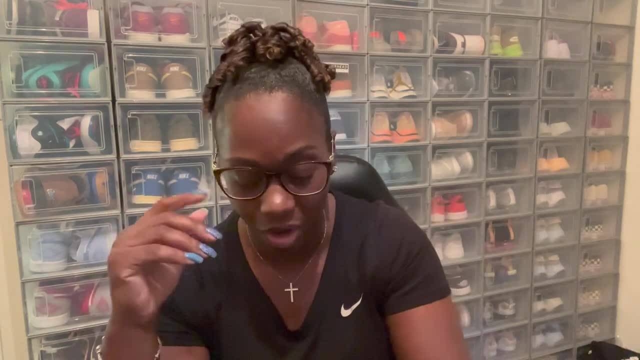 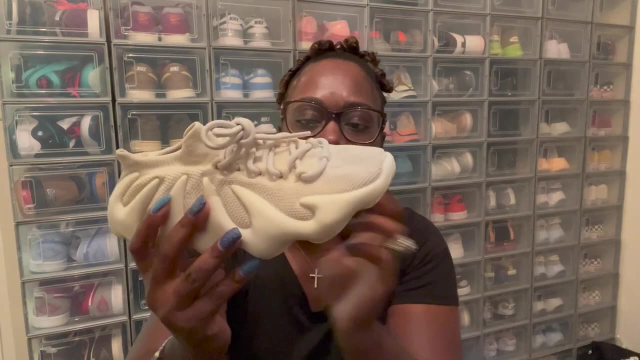 sure I can wear these with plenty more things. I love the cloud whites. They have these right here and yeah they- they do get dirty real quick. I mean you can see a little dirt going on my shoes because I wear these often, But I love them. I can go to a lot of stores. I. can go to a lot of stores. But I can go to a lot of stores. I can go to a lot of stores And, yeah, I can go to a lot of stores And yeah, that's what I'm talking about. I had a 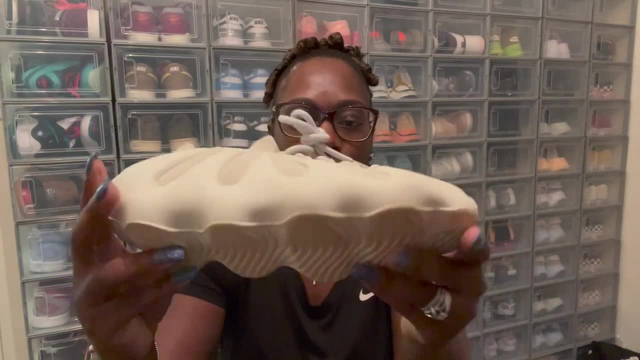 lot of clothes from myself, but I love them And I like to go to a lot of stores and I'll give you can see a little bit of dirt on the bottom, of course, from me walking around, but yeah, they, they got a little dirty. it's a little dirt specs here and there on the shoe, but i mean. 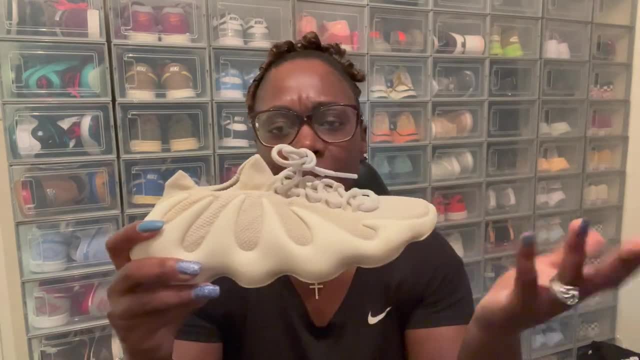 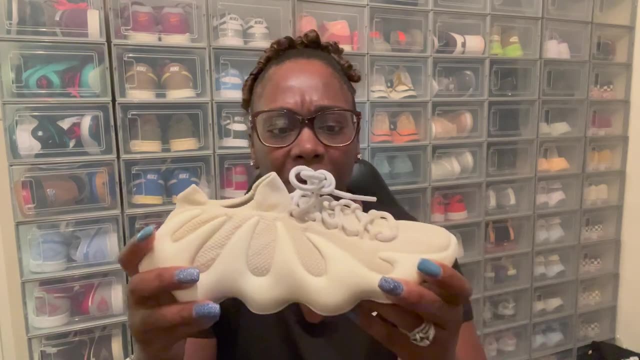 overall, i wouldn't say they get totally just messed up by you wearing them all the time, because i wear them a lot and they're not as bad as i thought they'd be, as they have red. some people say that they get horribly dirty, but i mean i i don't go wear mine in the dirt also, so they. 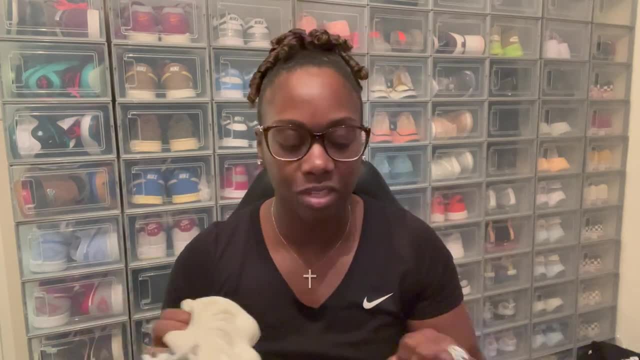 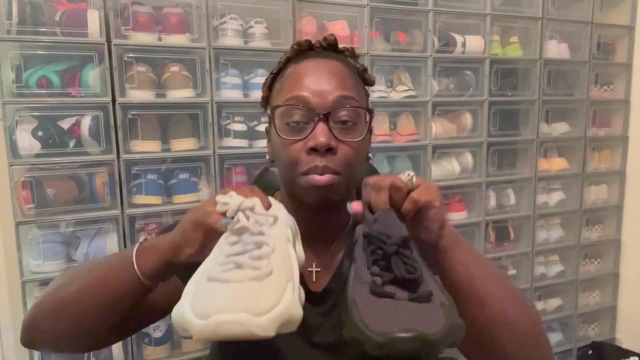 wasn't too bad. but yeah, this was the cloud whites, and then this was the dark slates. y'all let me know which color you think was the best: the cloud white or dark slates? i personally like both of them, but my best one as of now, i will go to the dark slates just because they're dark. now i have 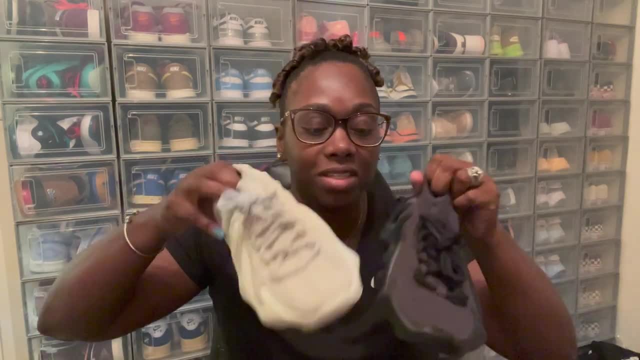 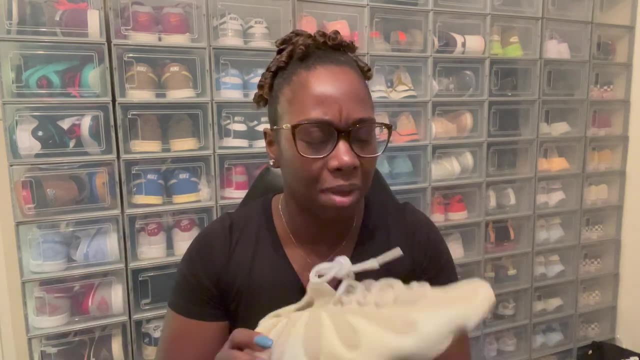 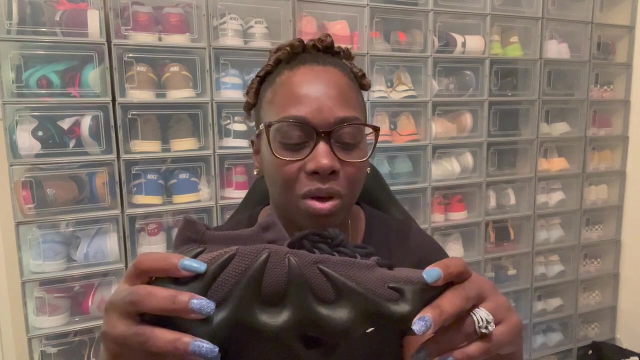 to worry about getting as dirty, but i love the cloud white so i can't. i can't really pick. i love them both, so it's totally a preference. i know they also came out on the 17th, but the dark slates was a resin. it was like a dark green colorway. i really wasn't feeling that colorway so i was like i'm not. 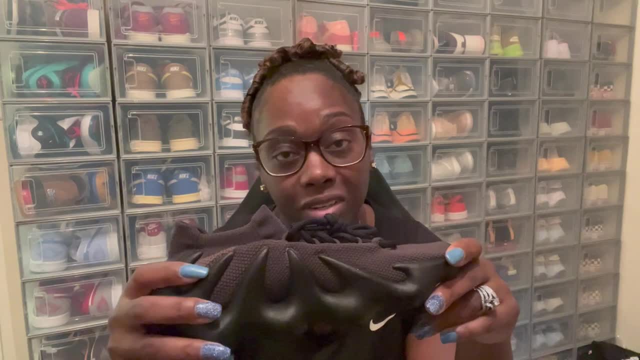 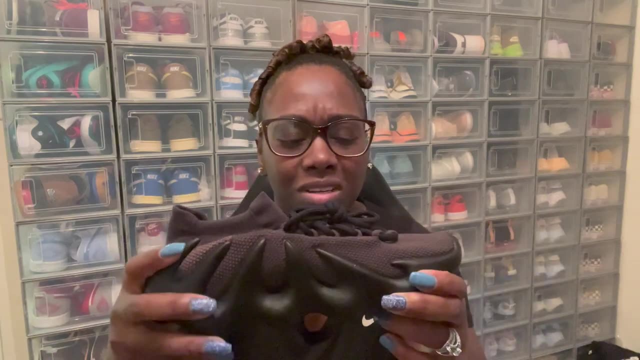 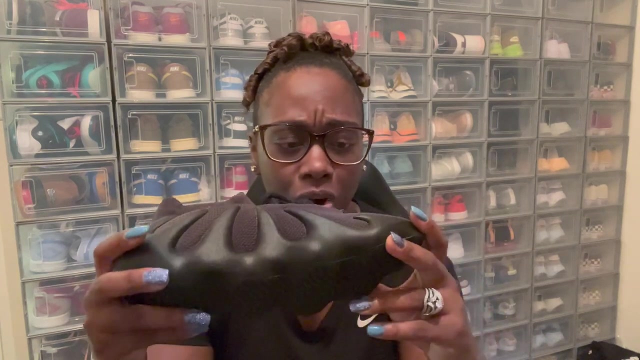 even going to try to get that one. i know some people said it is different, which it is, because it's real dark, like a military light green looking color, but i couldn't see myself with those right there, so i like had to go for these dark slates. i was so happy to be able to get them and, yeah, the overall. 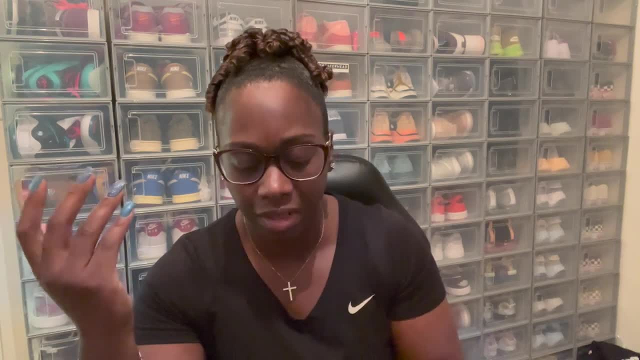 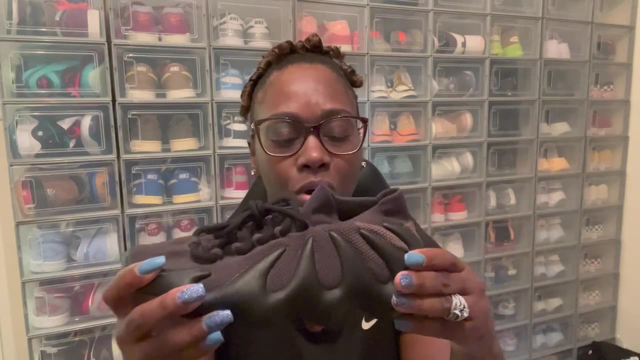 review of these shoes are that they're comfortable. i mean very comfortable shoe. once you put them on your shoes locked in, even though they don't have to boost on them, it doesn't even matter. they're comfortable, you can put them on, wear them all day, walk around all day and you've 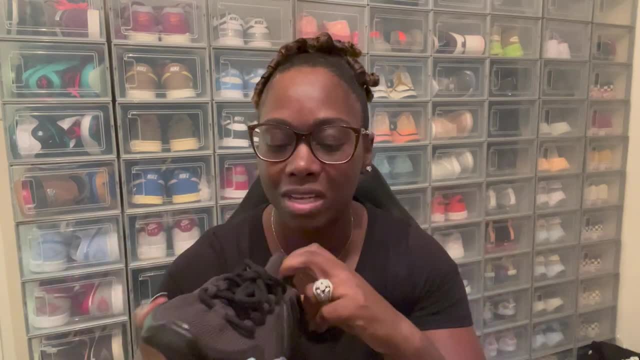 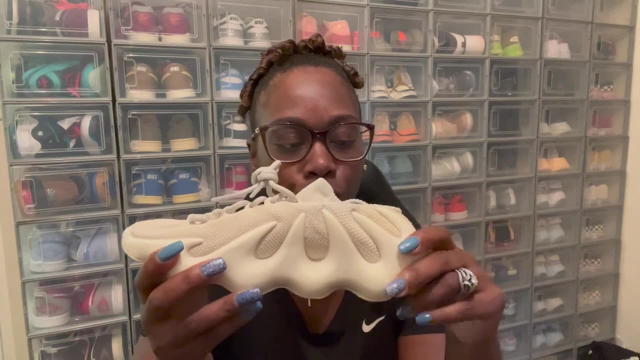 got your feet to be just fine, they won't hurt or nothing. uh, sizing wise, i usually go a half a size up. so on the cloud whites i got, i have a six and a half and they fit good and i have a little extra room in them. but unfortunately, in the dark slates i wasn't able to get a six and a half, so i had to. 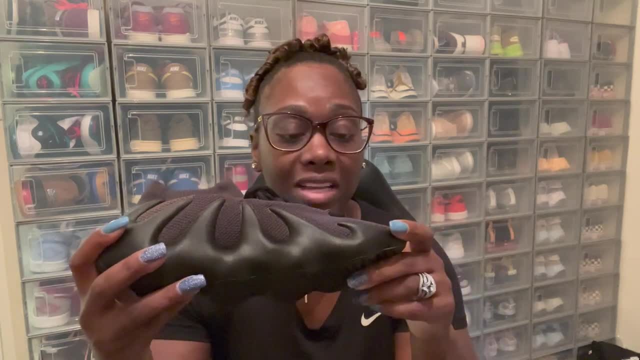 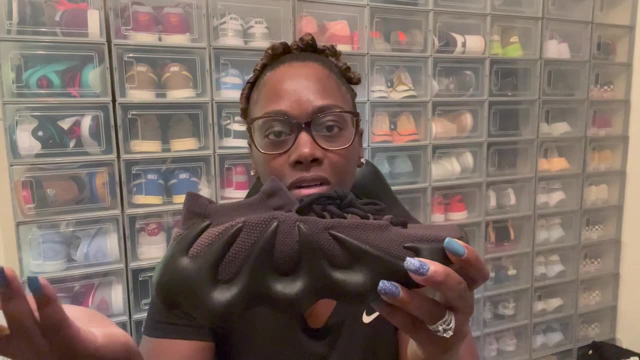 go with the six and they still fit perfectly also. so i guess it's totally up to what type of foot you have. if you have a thin foot- i mean a slim foot, and you should- you should be able to go either half a size up, or either you can stick to your true to size. it's totally up to you. 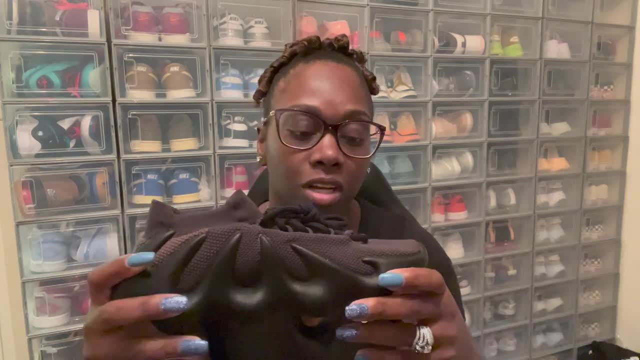 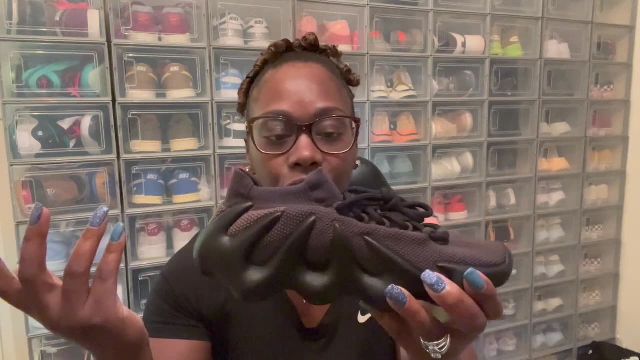 and the comfort of level of the way you like your uh shoes to feel. so i mean, like i said, i got six and a half in the cloud whites. they fit good. and then i got a six in these and they fit just fine also. so it's totally up to you. but um, that was my, that's my. you know what i gotta say about the? 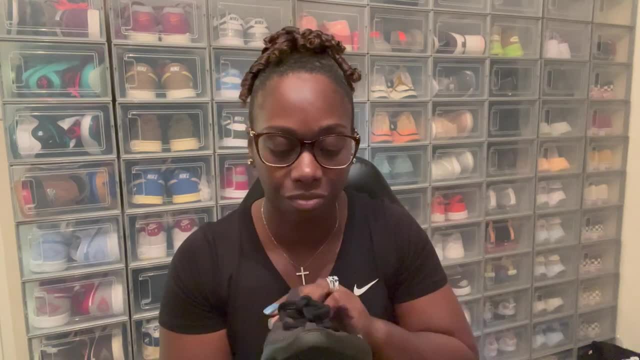 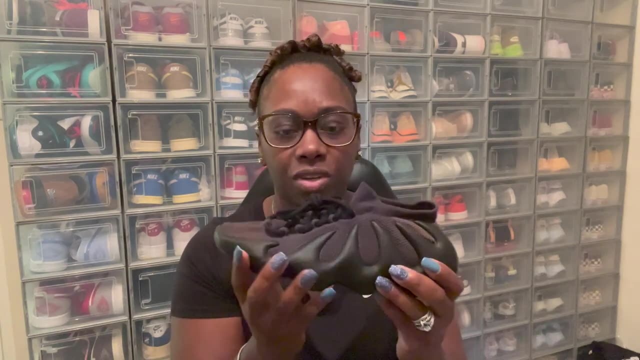 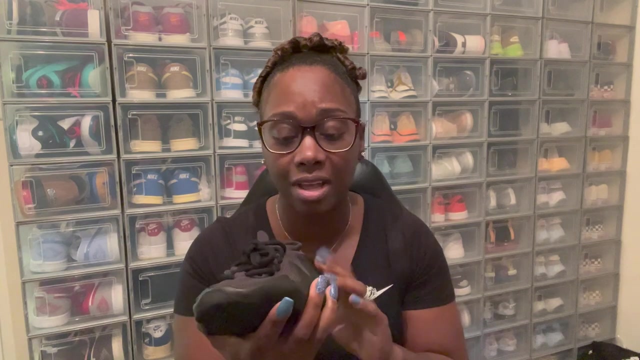 size- and i mean that's the best way i can put it- is totally up to your foot, unless you have a wide foot. now if you have a wide foot, i would say, go up a half a size just for that extra room, because it has that little extra room if you have wide feet. so but other than that, this shoe was a 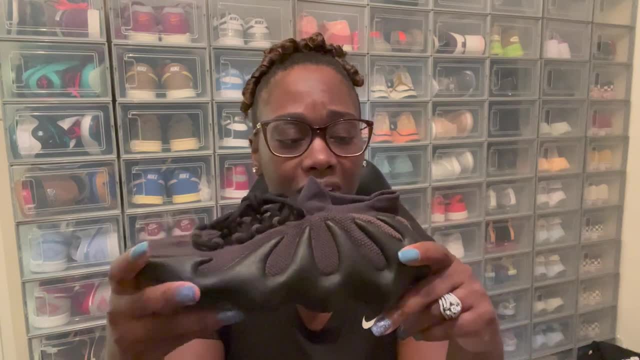 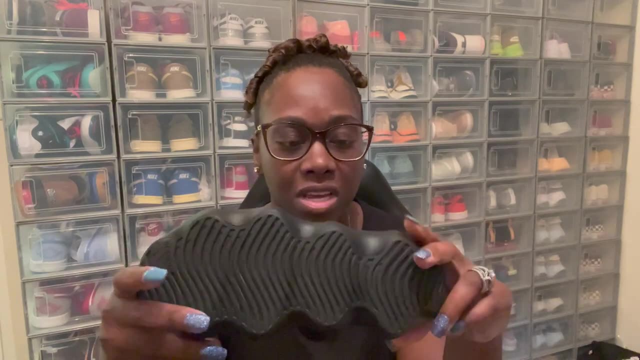 nice shoe that you could just grab to go anywhere, any, anytime, anywhere, you can dress it up, dress it down. i personally like to throw mine on and wear them to the gym, because it's a perfect gym shoe. um, i love the mesh and the salt, like material that clings to my feet, and they just, they, just. 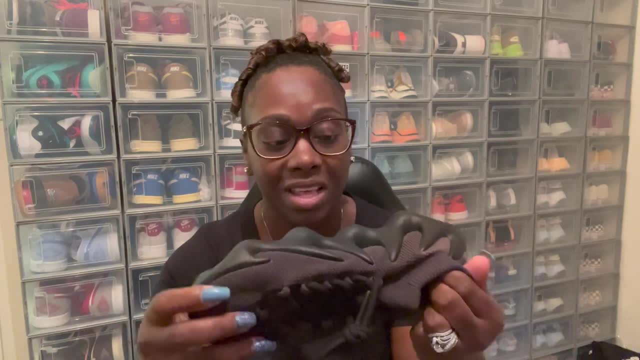 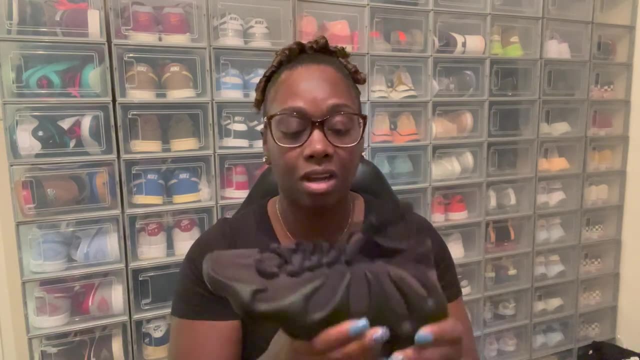 feel so comfortable when i have them on it's like you don't even realize you have them on, because that's how light and comfortable they feel. so, yeah, that's uh. this is it on the uh yeezy 450, uh dark slate. i mean y'all let me know down in the comments below. 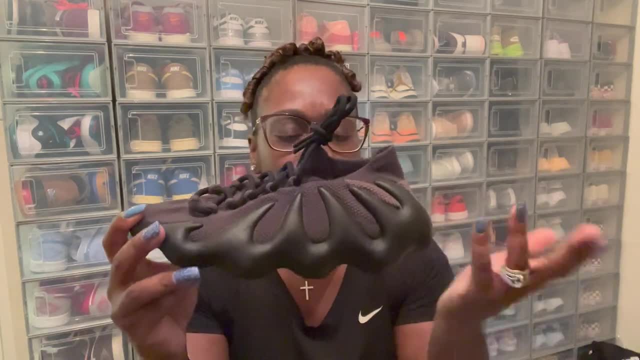 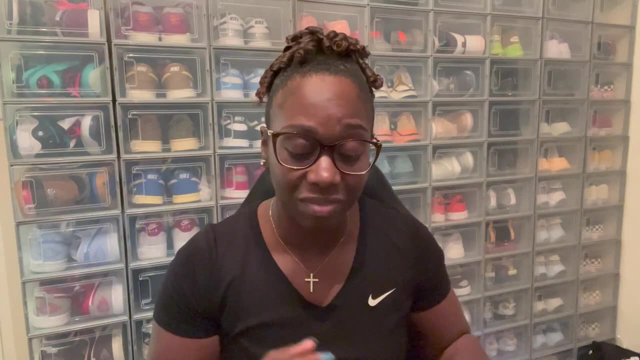 did you go for any one of the ones that came out on december 17th- the dark slate or the resin y'all? let me know which one you went for, if you went for any of them, or just let me know you don't even like them, period, like you might be like. why does people even like this shoe? but i mean, i was like 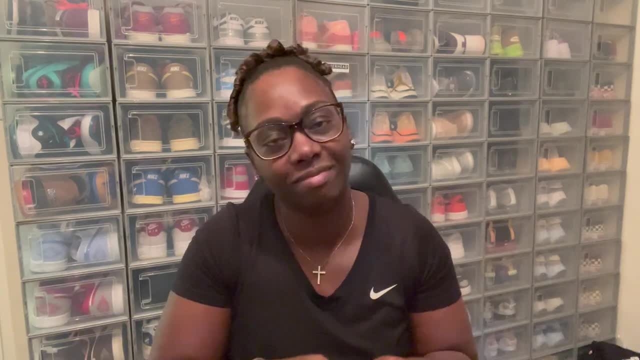 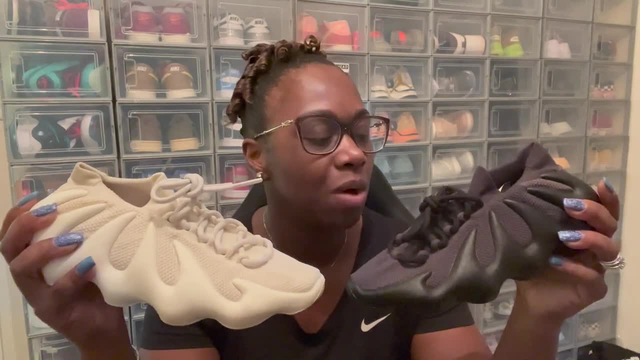 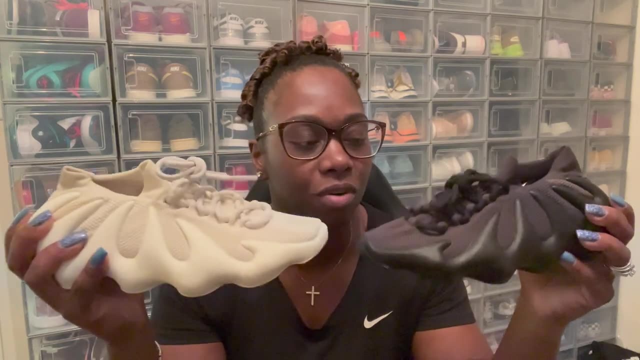 we got the cloud white yeezy 450s. i would say they got to be one of the top 10 yeezys of the year. both of them, they got to be in there. both of them have to be in that lineup somewhere because 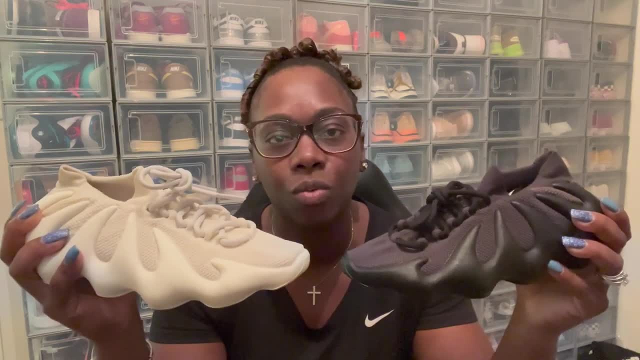 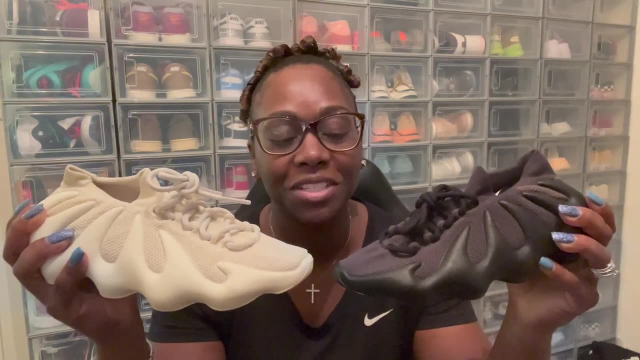 it's such a different shoe and i like the way they just look different and when you wear them they're going to draw attention and people going to be like: what is that you wearing? but you know that they they draw your attention, so you know there must be something about the shoe. 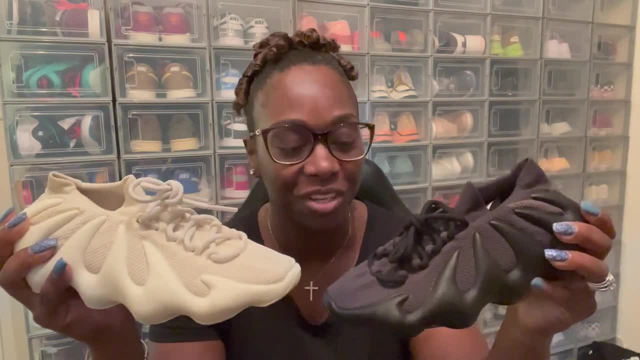 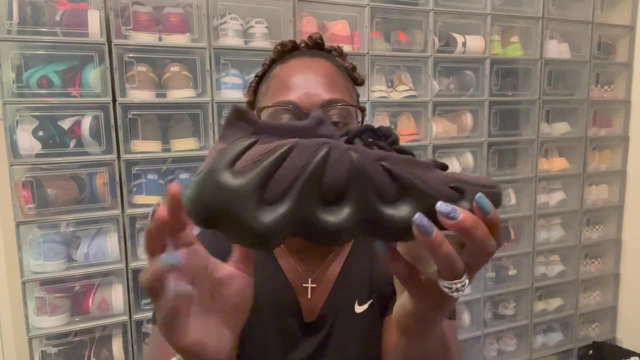 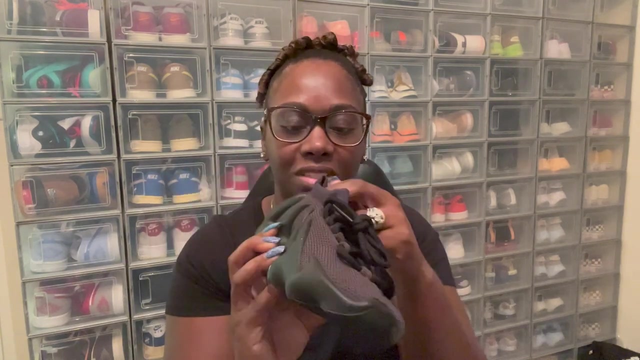 whether they like them or whether they hate them, that they look down at your foot. so but yeah, that's all i got for y'all today. yeezy, 450 dark slate. let me give you a 350 of the dark slate, all right, and yeah, um, continue to like and subscribe, continue to follow your girl on. 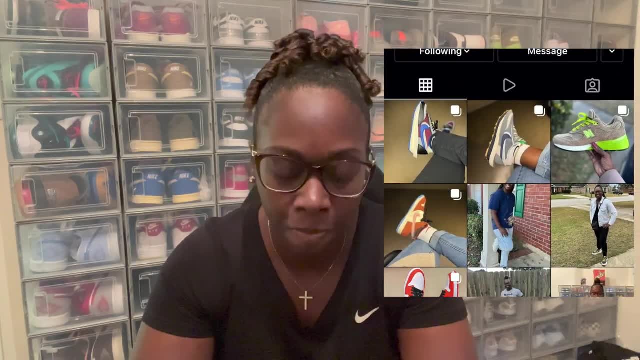 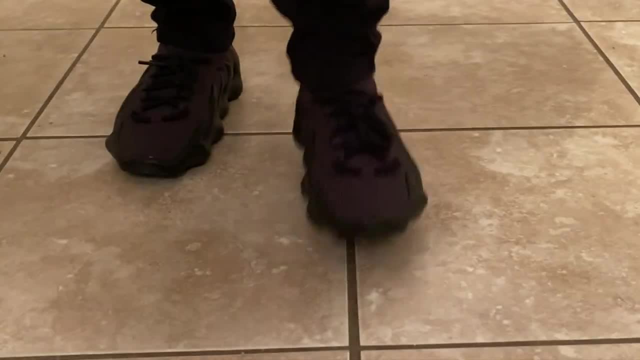 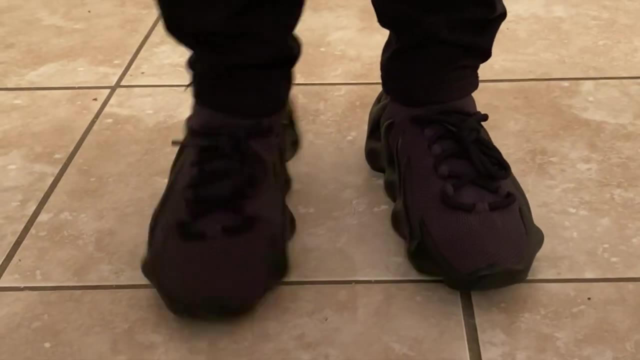 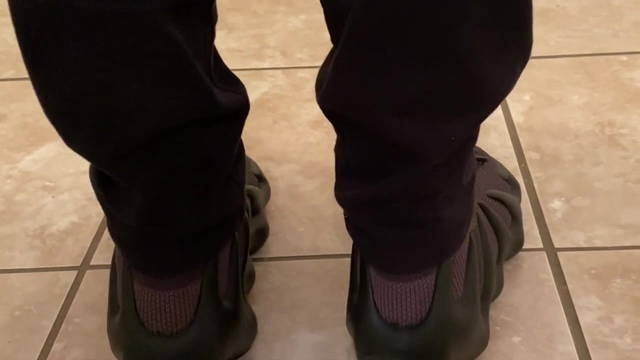 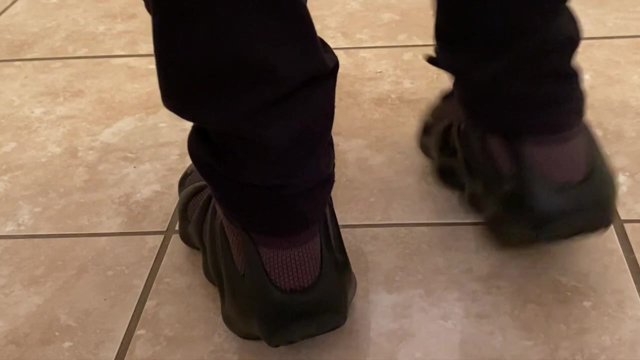 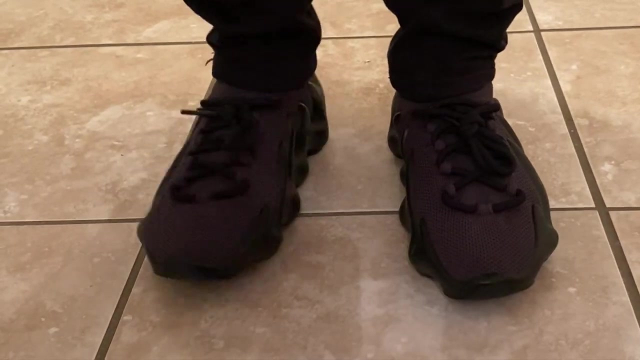 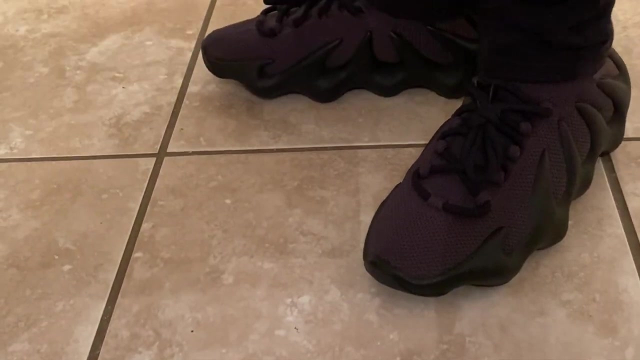 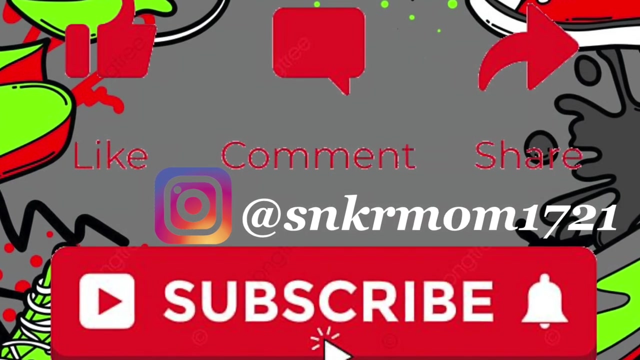 instagram at sneaker mom 1721. and yeah, that's all i got for y'all, but hey, until the next time it's your girl, sneaker mom, peace out. so, so, so, so, so so. 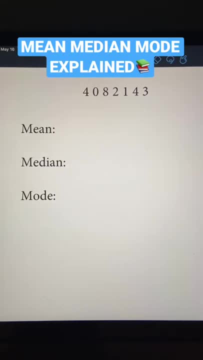 This is how to calculate the mean median and the mode for any type of data set. So the first thing you want to do is write these numbers in order. So it's just going to be 0,, 1,, 2,, 3,, 4,. 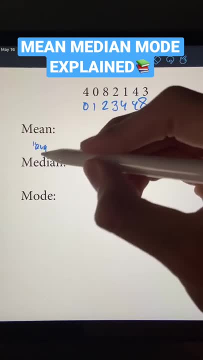 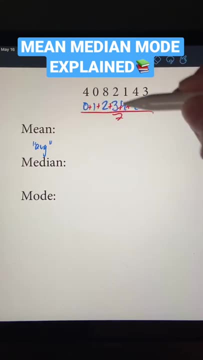 4, 8.. Okay, anytime, you want the mean, you want the average? Okay, and you can find the average by adding all of the numbers up and then dividing by however many numbers there are. So there's seven numbers you divide by seven. So if you work this out, it's going to be 22 over seven. So median is 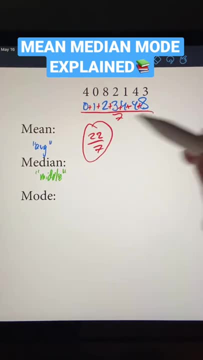 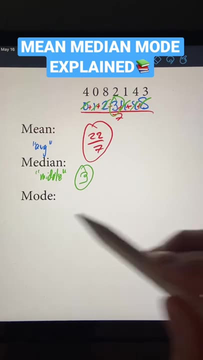 just fancy word for middle. So you want to find the middle number. So we can do that just by crossing out the ends until we only have one number left, which is three, which is our median And mode. the way you can find the mode is: think of most, which is the number that appears, the